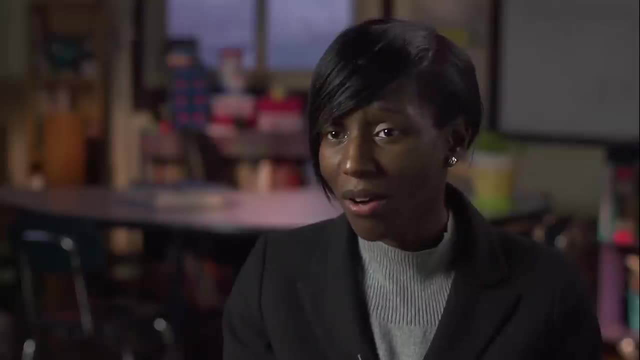 When you borrow, what do you borrow for? You know why do you borrow So literally? you have students, Students, just you know, crossing out numbers, yet they don't know why. 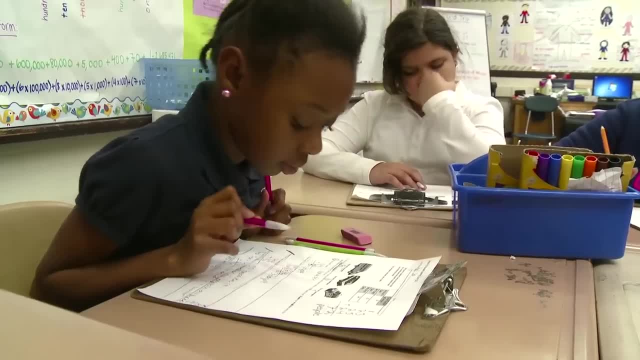 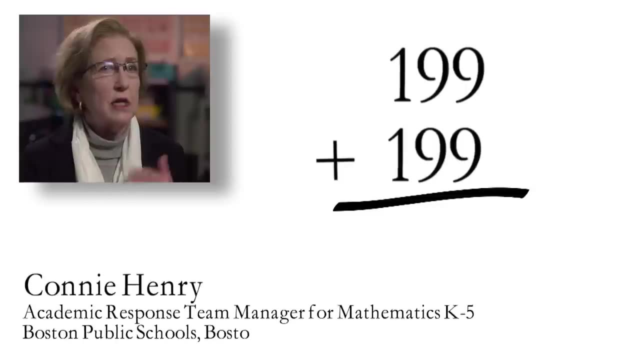 Or why do they carry? You know why do you carry a 1?? What does a 1 mean? Is it a 10? Is it a 1?? If you think about the problem: 199,, 199 plus 199,. 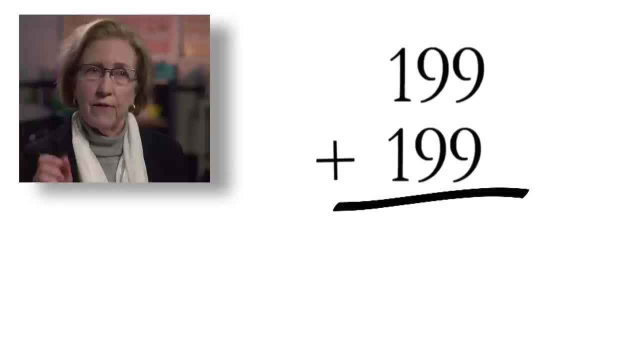 you can set it up as a standard algorithm. You can line them up very neatly. You can go 9 plus 9 because you're taught to add the 1's first and do it, and then make another little mark for the 1 that you carry from 18,. 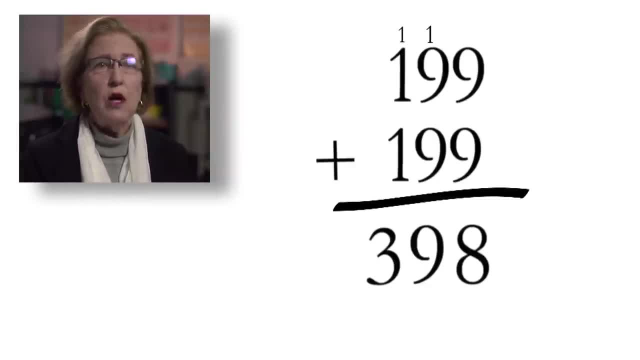 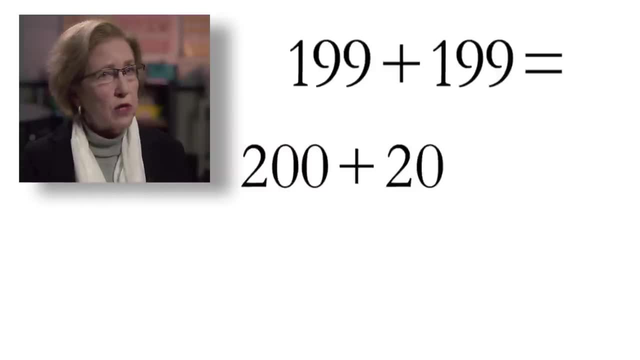 which isn't actually a 1,, it's a 10.. Or you can think flexibly: 199, 199 plus 199.. Well, I know 200 and 200 is 400, and I need to take away 2. 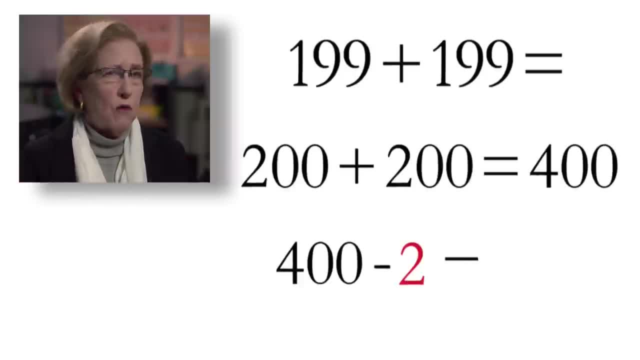 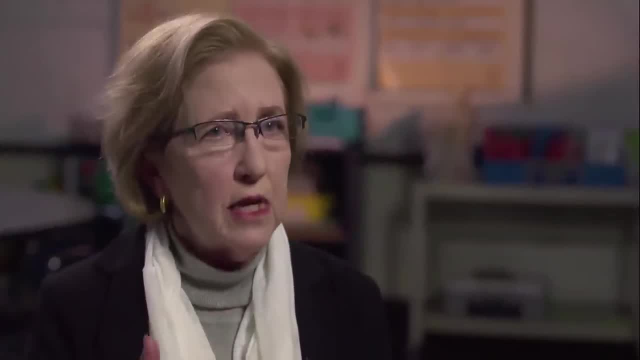 because it's only 199 in each case. Oh, the answer is 398.. And that is the kind of flexibility, the kind of thinking that you want to encourage. If you think about 12,, if you think about 12 divided by 3,. 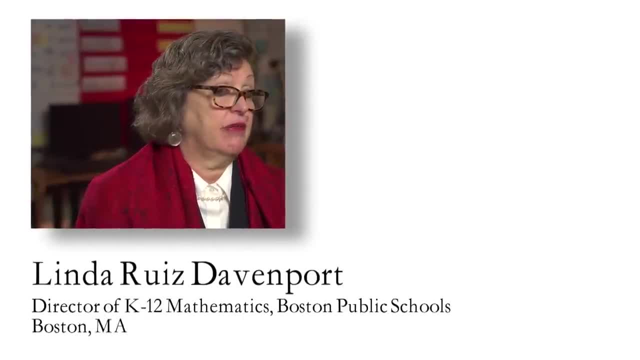 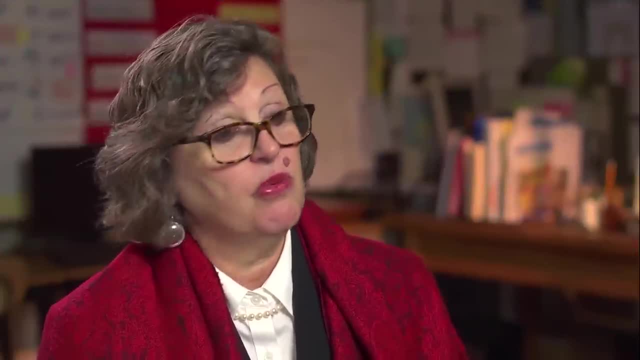 what you're really asking is how many 3's are there in 12?? So if you have a fraction division problem- for instance, 1 half divided by 1 fourth- really what you're asking is how many 1 fourths are there in 1 half? 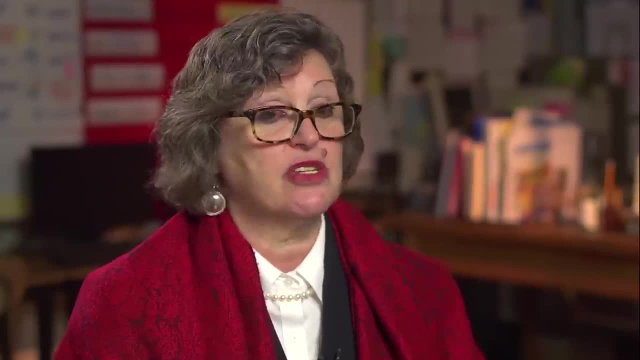 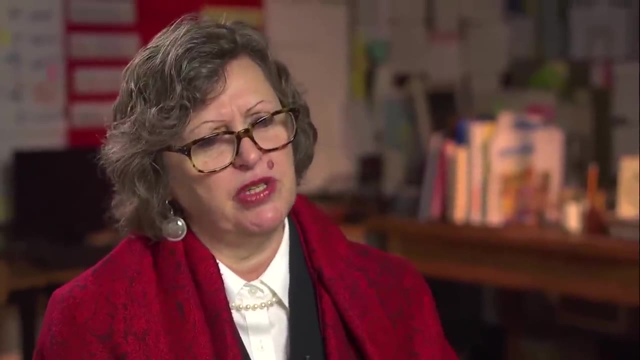 And the answer is simple. It's 2, because you know what these fractions look like And you can say there are two, 1, fourths in a half. The answer is 2.. And so it makes sense, not only from a point of view of what division means, but also. 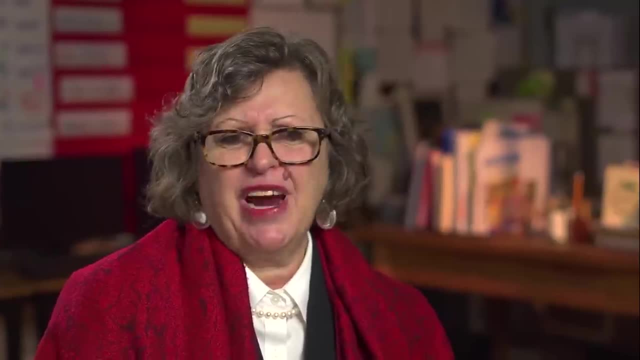 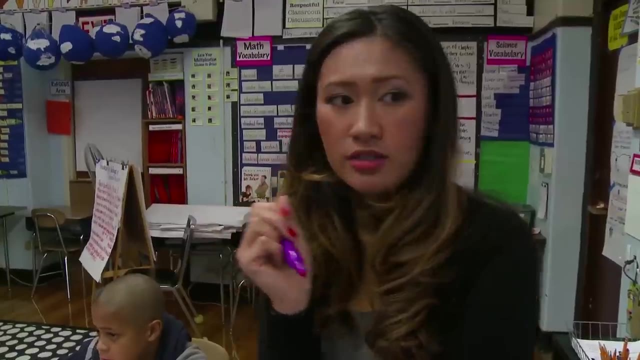 it helps address the mystery. It's a mystery of why, when you divide a fraction less than 1 by a fraction less than 1, you can get a number that's bigger than either of those fractions- More or less than 32?, If you like, do 32 times 1 tenth. I mean 1 whole. it would be 32..